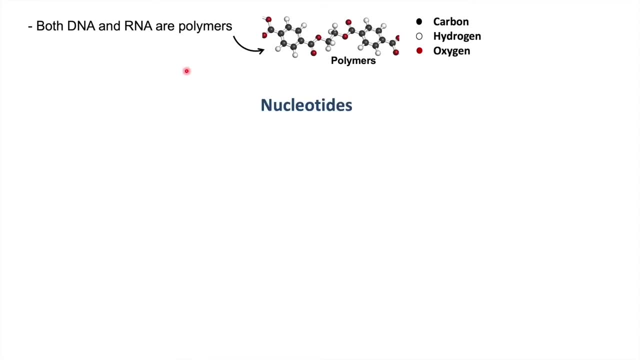 comes to both DNA and RNA. there are actually two materials in families: DNA, rna. these monomers are called nucleotides, and nucleotide which makes up dna is called deoxynucleotide, which contains a deoxy ribose sugar molecule, which is a pentose ring, a five carbon ring. 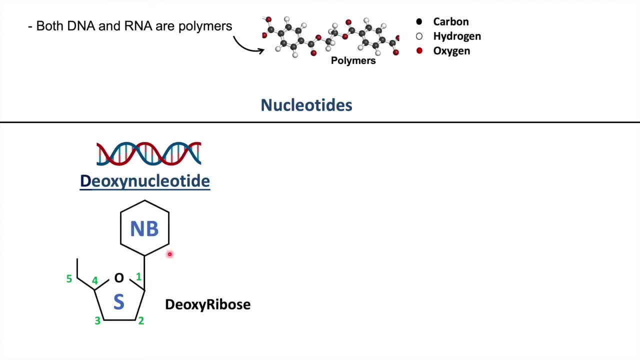 and it also contains a nitrogenous base which is attached to carbon. one position of the pentose ring, and it also contains a phosphate group which is attached to carbon. 5 position of the pentose ring, which is located outside the pentose ring. now the nucleotide which 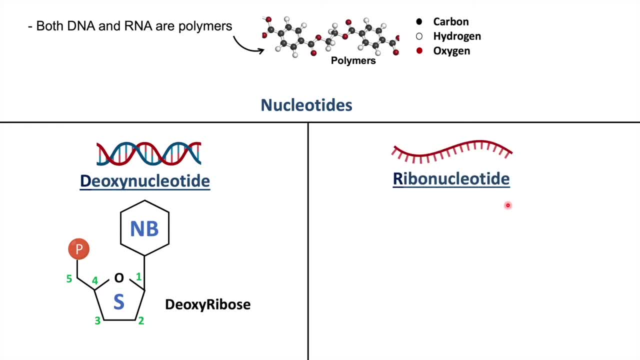 makes up rna is called ribonucleotide and it contains a ribose sugar which is again a pentose ring, and it also contains a nitrogenous base which is attached to carbon one position and a phosphate ring which is attached to carbon 5 position of the sugar molecule. so the difference between these two sugar molecules, that is, ribose and deoxyribose, is: ribose sugar has two hydroxyl group, which is attached to carbon 2 and carbon 3 position of the pentose ring, whereas deoxyribose has only one hydroxyl group, which is 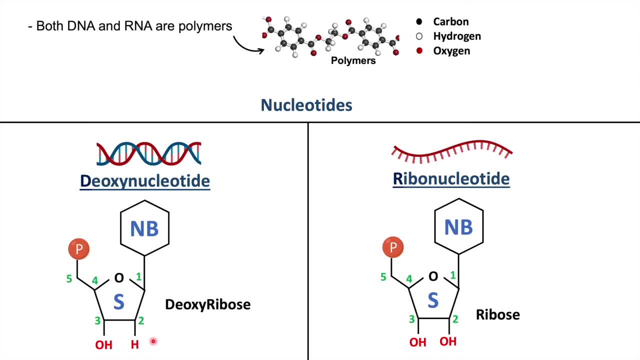 attached to carbon 2 position and therefore it is called deoxyribose, because it is missing a hydroxyl group here on carbon 2 position. so basically, nucleotides contain a sugar molecule, a nitrogenous base and a phosphate group. so now let's look more. let's look. 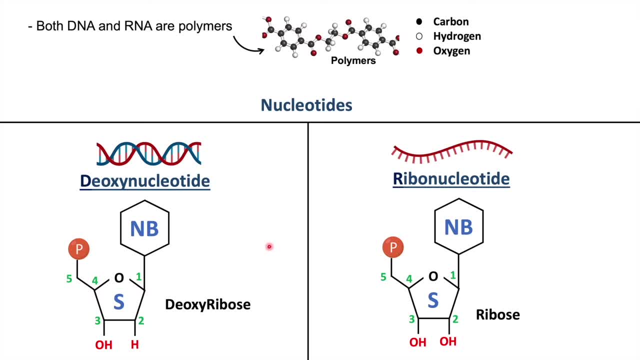 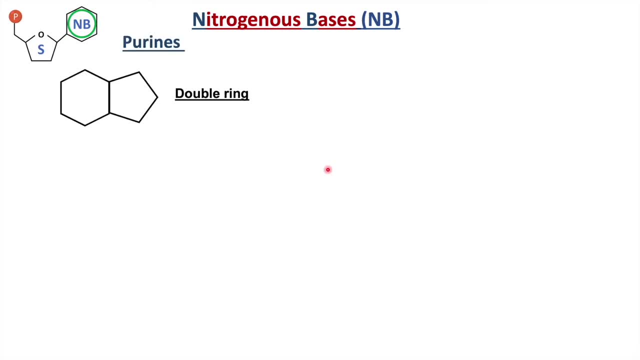 at more of the nucleotides in more detail about a nitrogenous base. so there are basically two types of nitrogenous base. one is called purines, which is a double member, a double ring. one is six carbon ring and another is five carbon ring, now the uh. the second uh nitrogenous base is called pyrimidines and which is only a six carbon ring. 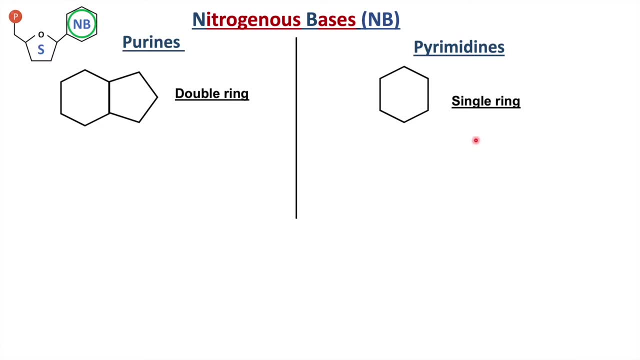 so that is. therefore, it is a single ring. now, the way to remember, uh, whether purine has a double ring or pyrimidine has a single ring, there is one way to remember- is because purine it has a shorter name but it has a larger structure. 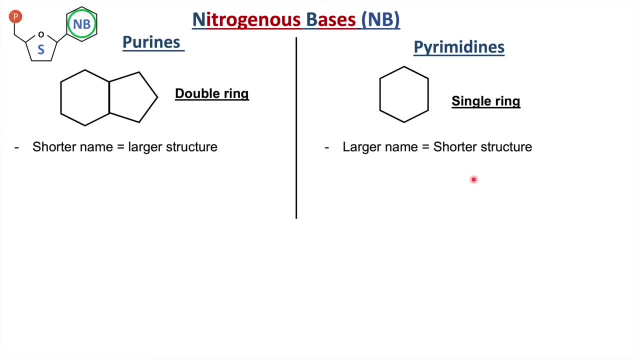 at the same time with pyrimidines. it has a larger name but it has a shorter structure. so this is kind of very a nice way to remember, one way to remember that you know, purine has a shorter name but has a larger structure because it has a six carbon ring and a five carbon ring, whereas pyramid has a larger name and the shorter. 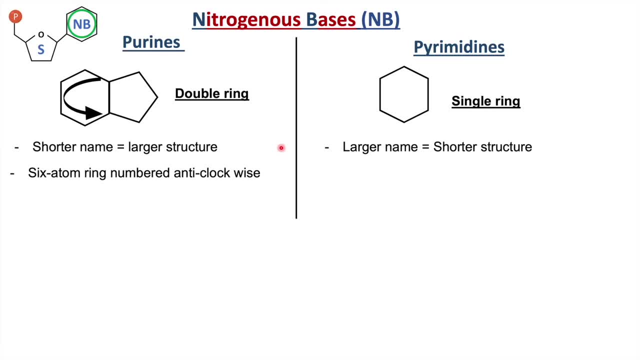 structure. now, the other thing about purines and pyramids are the six atom ring or the six carbon ring in purines are number anti-clockwise manner, whereas six carbon ring in pyramidines are numbered. Now, purines includes adenine and guanine, whereas pyrimidines are thiamine, uracil and cytosine. 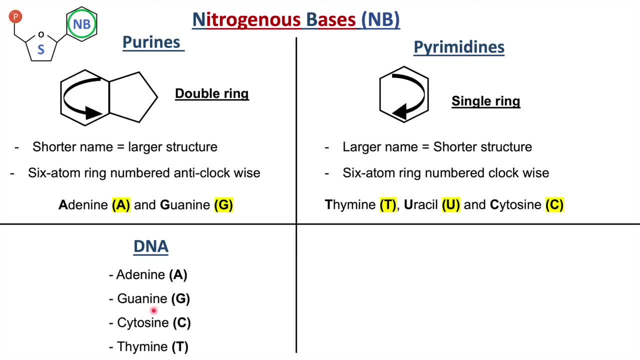 So DNA contains adenine, guanine, cytosine and thiamine, whereas RNA contains adenine, guanine, cytosine and uracil. So the difference between two is only DNA has a thiamine, whereas RNA has a uracil. 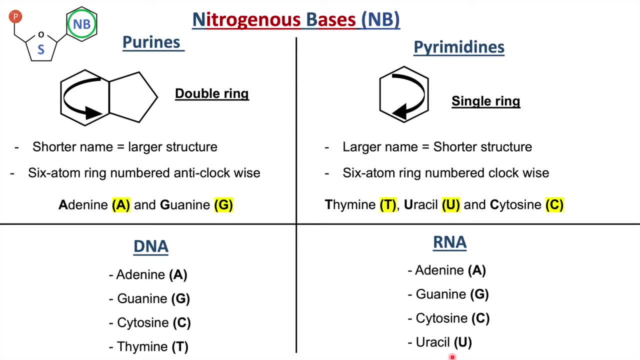 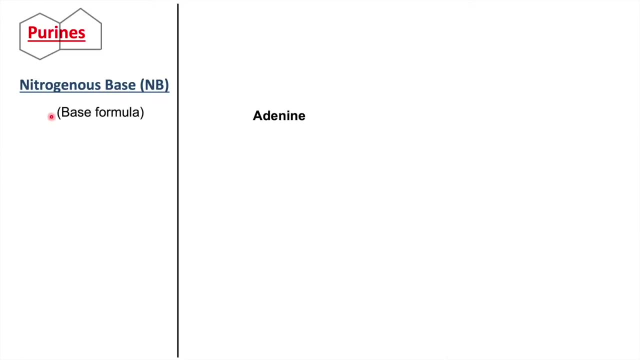 So that is the important difference which everyone, I guess, needs to remember. Okay, So now let's talk about a little bit in detail about purines and pyrimidines. So purines, like I suggest it has a shorter name and a larger structure. 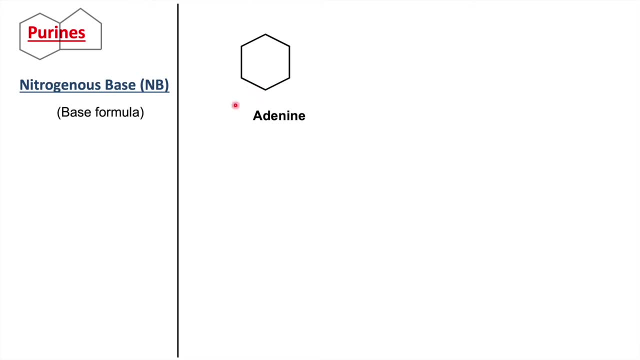 So the basic structure of purines, as you can see here, it has one six membered carbon ring and second is five membered carbon ring. So, if you remember, The six six carbon ring of purine is numbered anti-clockwise manner. So let's number this ring. 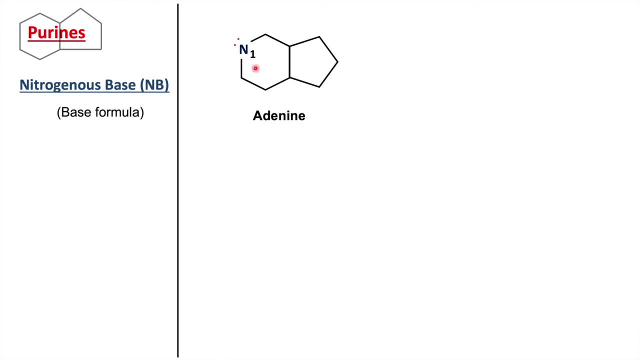 So on first position we have nitrogen group attached and there is also another second nitrogen group, nitrogen atom, which is which is on third position. So that means Okay, Okay. So for the five carbon ring there are two nitrogen atom and four carbon atoms. 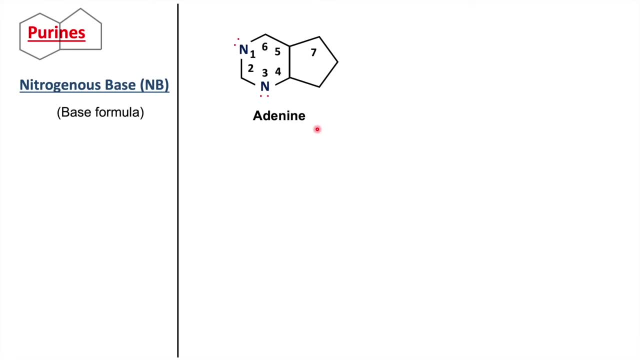 Now on the on the five carbon ring. the five carbon ring also has two nitrogen atoms, which is at position seven and position nine. So here there is a hydrogen atom attached to nitrogen, and where there is no hydrogen, that means that means there is a lone pair electron of nitrogen. 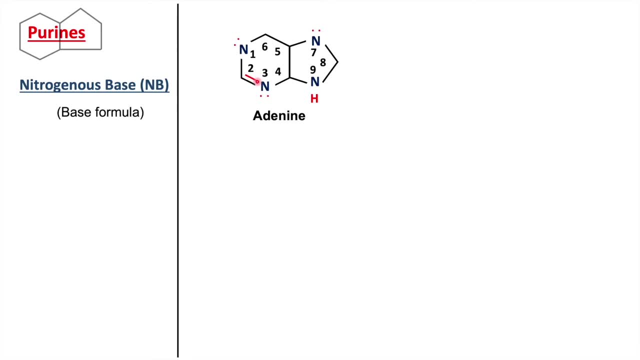 now it also has a double bond between position 2 and 3, position 4 and 5 and position 7 and 8. so this is the basic structure of purines. so this is guanine, which is also the same basic structure of purines. 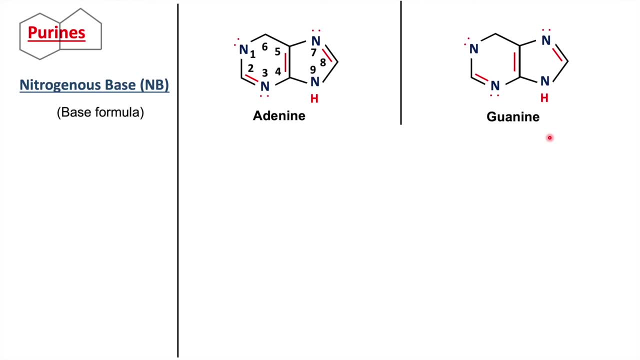 now. now let's look at the difference between adenine and guanine. so the one difference is: there is an additional double bond in adenine between position 1 and carbon 6. now there is a NH2 group which is attached to carbon 6 position of adenine. 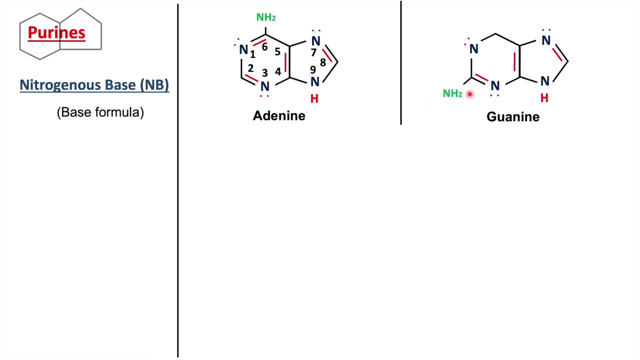 whereas in guanine there is a NH2 group which is attached to carbon 2 position of 6 carbon ring in guanine. so this is the difference between adenine and guanine. now let's look at the difference between adenine and guanine. and another important difference in guanine is there is a carbonyl group which is attached to carbon 6 position of 6 member ring. 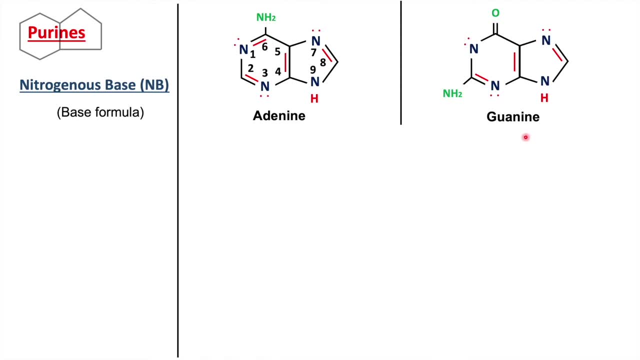 so this is the structure of adenine and guanine. so now, when the sugar molecule is attached to adenine or, suppose, guanine, it is important to remember that sugar molecule can be only attached to guanine by斧 9 of the five member ring, which is called a N9 position. 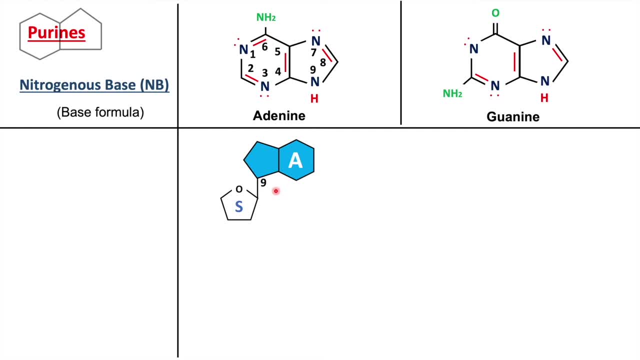 where N9 located is. this N9 is the 9th position of nitrogen atom in purine ring. so this is very important, guys. you need to記得. sugar molecule can be only attached to the N9 position of the purine ring. next matter is the fallout on the bottom in mid dameric. 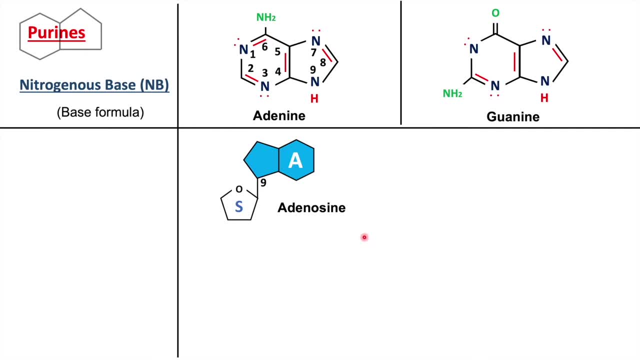 attached to adenine, it is called adenosine. Similarly, when the sugar molecule is attached to guanine at N9 position of nitrogen atom, it is called guanosine. And both these attachment of sugar to adenine or guanine are called nucleosides. So nucleosides basically. they. 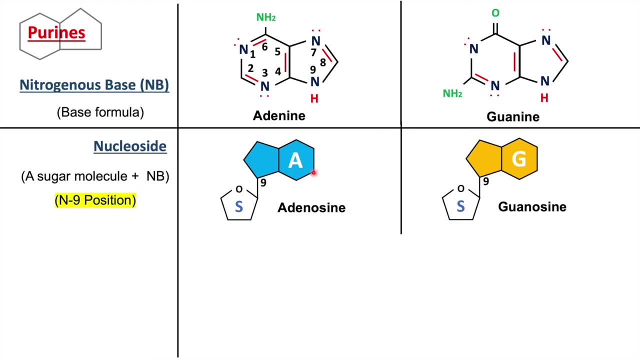 are just a sugar molecule which is attached to nitrogenous base. So this is nitrogenous base and then when you add another sugar molecule it becomes nucleoside And most importantly- I am emphasizing again that it is sugar molecule- is attached at N9 position of the purine ring. 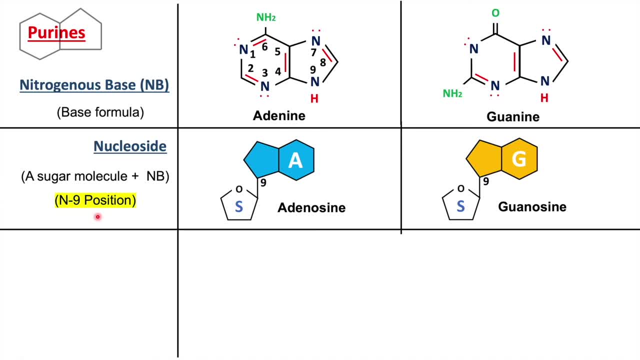 Now, lastly, when the phosphate group is attached to the sugar molecule, it becomes adenylate and it is, and in this structure, like I showed before, that the combination of a phosphate group and a sugar molecule and a nitrogenous base is called nucleotide. So, again, when the phosphate group is attached to nucleoside, it 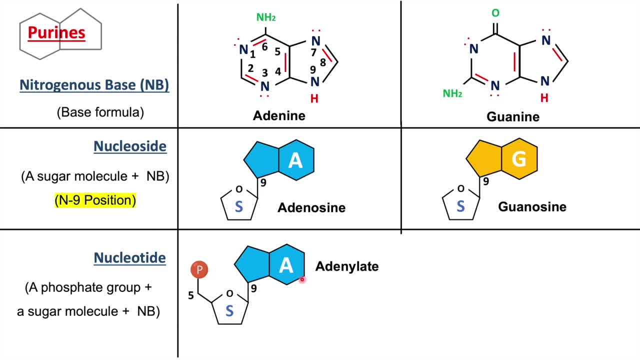 becomes nucleotide. So here in this case it is called adenylate, but alternatively you could also called like you can also name this nucleoside, which can be called adenosine, because this is adenosine. this is the basic structure of adenosine, and the phosphate group is attached. 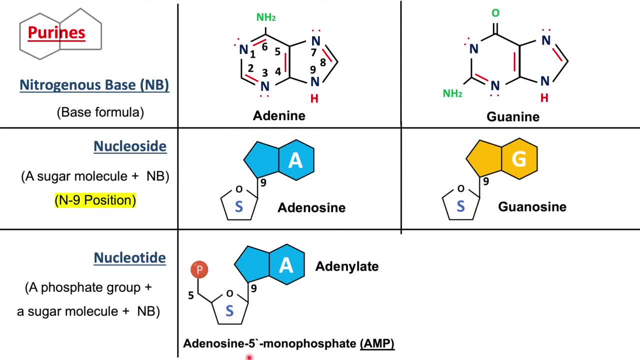 to carbon 5 position of the sugar molecule. therefore it is called 5 prime monophosphate. So therefore it is called adenosine 5 prime monophosphate is called a another one, but you could also call it adenosine 5. 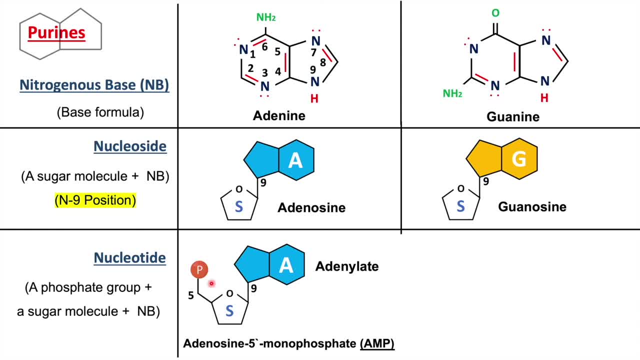 monophosphate, that is AMP. and if there is 2 phosphate group attached to the sugar, it will. it will be called adenosine diphosphate. if there are 3 phosphate, it will be called adenosine trifosphate. That means ADP or ATP. now, similarly, when the phosphate group is, 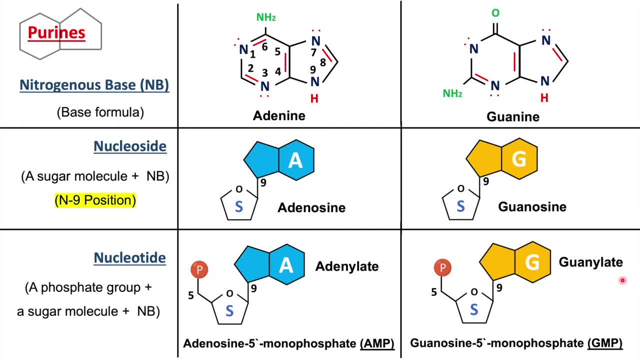 it is called gonelate and alternatively it is also called gonosine 5 monophosphate. so again, just to clarify: this is our nitrogenous base and when the sugar molecule is attached to nitrogenous base it becomes nucleoside. and when you when and when the phosphate group is attached. 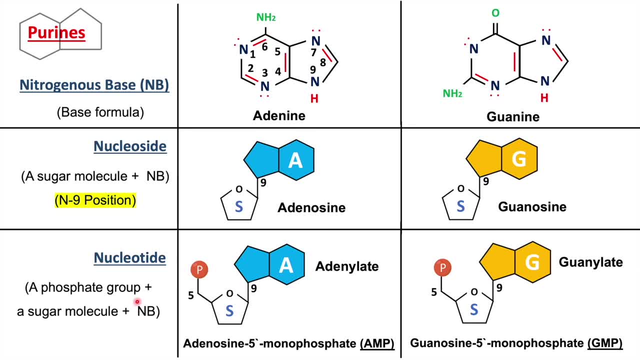 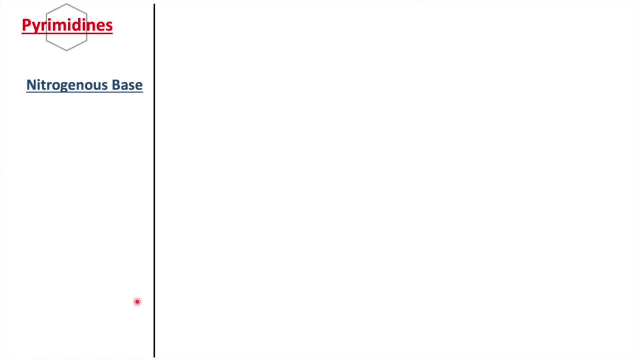 to nucleoside, it eventually becomes nucleotide. so this is very important, guys, to remember. now let's look into pyrimidines. so, like i said, pyrimidine has a longer name but a shorter structure, so pyrimidine contains six carbon ring. and let's look into the basic structure of 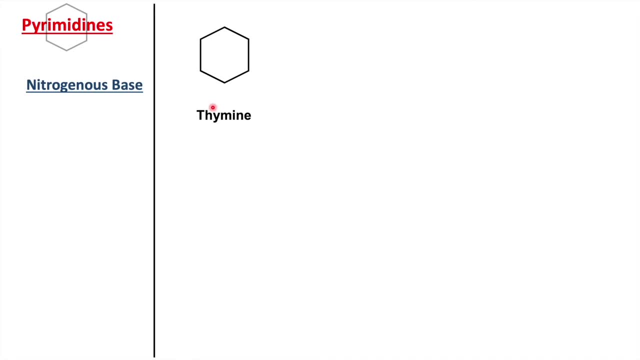 all three pyrimidines, those are thiamine, cytosine and uracil. so so, if you remember the, the six member ring of the of pyrids is pt Of Pyrimidine, which is the, the вообщеleme of pyridine. 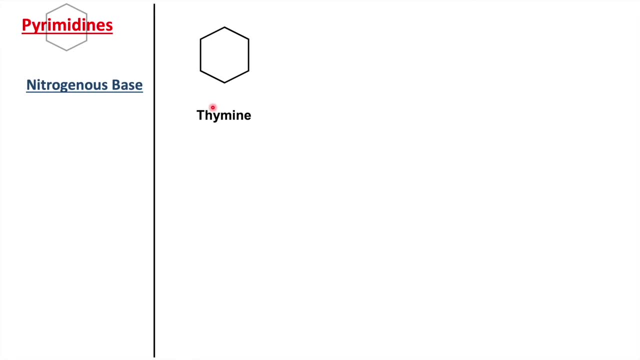 is numbered clockwise manner, so let's number this ring. so this is the carbon one position where nitrogen atom is attached, carbon two and there is another nitrogen atom at carbon three position and four, five, six. so basically there are two nitrogen nitrogen atoms and four carbon atoms in pyrimidine ring and 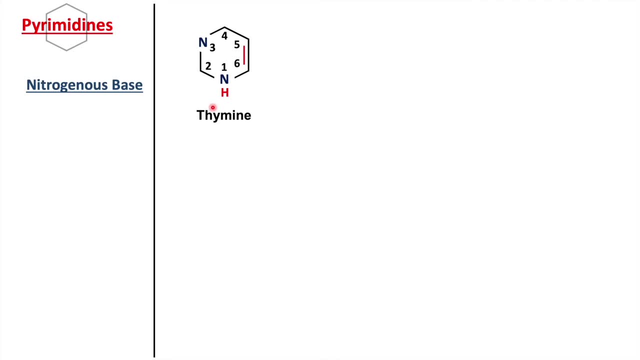 there is a double bond between carbon five and carbon six. so this is the basic structure: two nitrogen atoms and one double bond between carbon five and six. so now let's look at the difference between these three: thymine, cytosine and uracil. so the one common, one common group which is attached to carbon two. 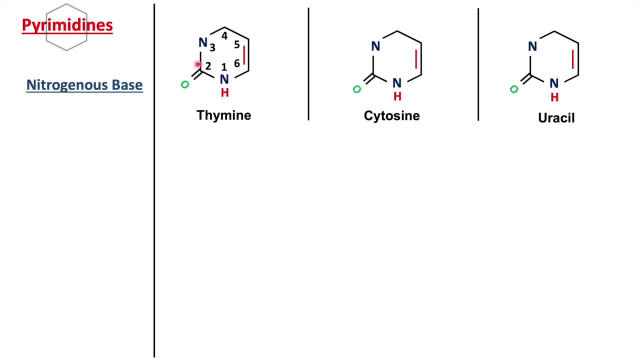 position is the carbonyl group. so carbonyl group is attached to carbon. two position: in all time, in all three pyrimidines, that is, thymine, cytosine and uracil. now the difference is there is a hydrogen group, hydrogen atom, on thymine and uracil. on position three and the other difference is there: 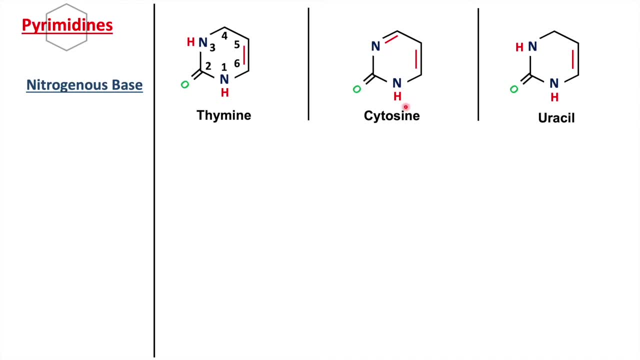 is a double bond between position three and four of cytosine and, most importantly, there is a carbonyl group on thymine and uracil on position four. so this, both thymine and uracil, they look very similar at this point. 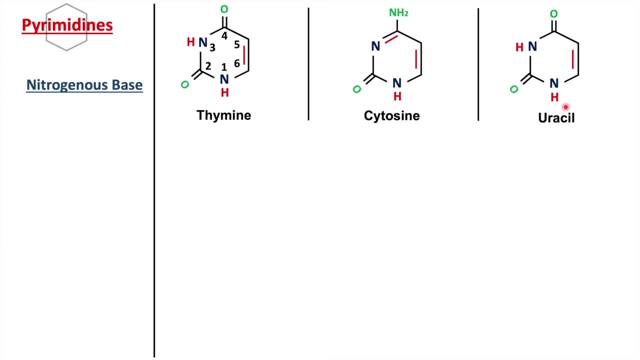 they are very similar. the only difference is that there is a methyl group attached to carbon five on thymine, whereas there is no methyl group on uracil in carbon five position. so this is the only difference between thymine and uracil. and with cytosine there is a NH2 group, which is which is attached to 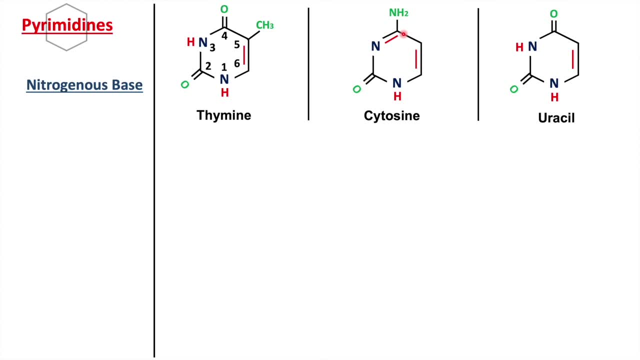 carbon four position. again, this is not very important to remember the structure of purines and pyrimidines, so you don't really need to follow this. but most important thing to follow is the transformation of nitrogen base to nucleoside, to nucleotide. so let's, let's see how nitrogen base is now transformed. 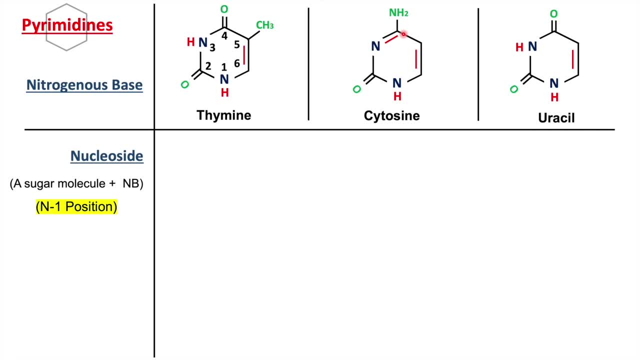 into nucleoside. so, like we saw before, that nucleoside are basically attachment of sugar molecule to the nitrogenous base. so when the sugar molecule is attached to nitrogen base, the important thing to remember here, unlike of purines, that the sugar molecule is attached to. 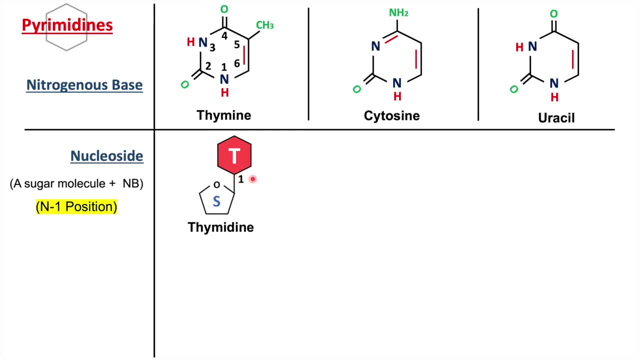 N 1 position of perimidine ring. that is the N 1, that is the position one of nitrogen atom in six member ring. so when the sugar molecule is attached, attached to thiamine, it becomes thymidine and that is its nucleoside, comes thymidine and that is its. 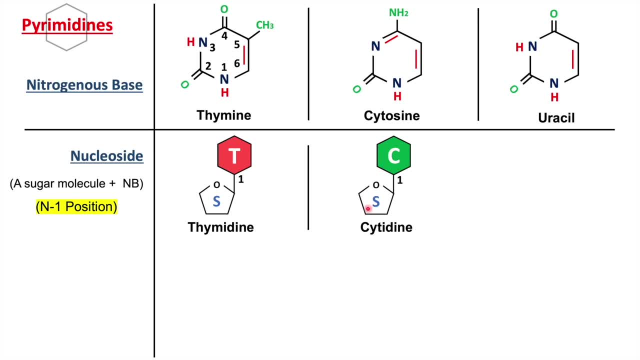 nucleoside, now when it is attached. when the sugar molecule is attached to cytosine, it becomes cytidine. now when the sugar molecule is attached to uracil, it becomes uridine. and lastly, when the phosphate group is attached to nucleoside, it becomes nucleotide. and when the 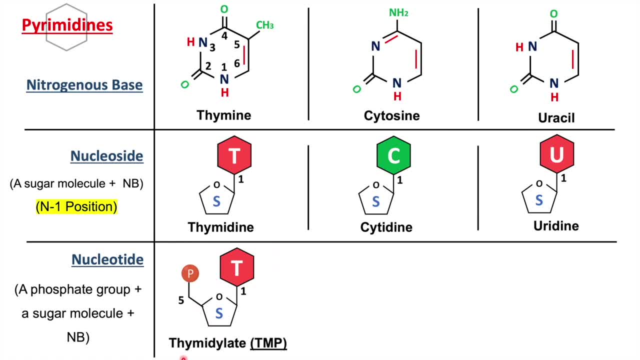 phosphate group is attached to thymidine, it becomes thymidylate and alternatively, it is also called as thymidine 5 monophosphate. therefore, it is also called as tmp and in case of cytidine, it becomes cytidylate and cytidine. 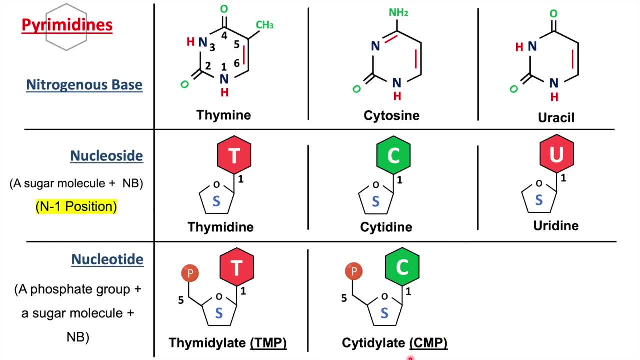 5 monophosphate, that is cmp. and when the phosphate group is attached to uridine it becomes uridylate and it is also called as uridine 5 monophosphate, that is ump. so again, the transformation from nitrogen base to nucleoside, to nucleotide, is important to remember here. 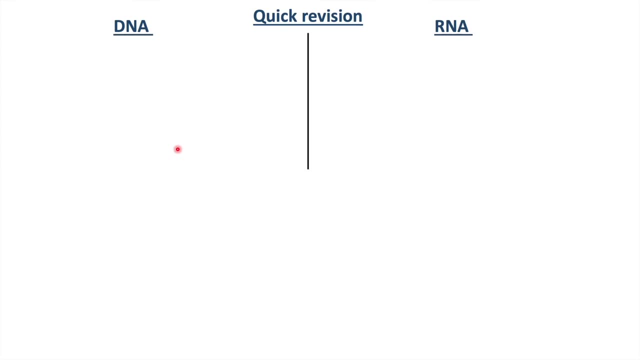 so just a quick, uh, just a quick revision. um so dna? uh, like we saw, dna is a double stranded molecule, whereas rna is a single stranded. dna is deoxyribose sugar. it is deoxyribose sugar because it lacks hydroxyl group. on position. 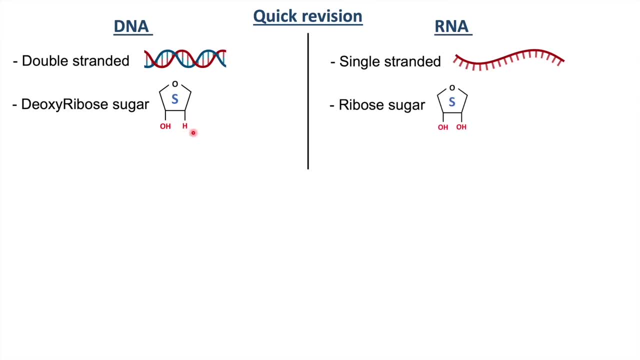 two of carbon atoms and ribose sugar, which has two hydroxyl group. now dna is located inside the nucleus, whereas rna is located outside the nucleus. dna is important in storing genetic information, whereas rna is important in transferring genetic information, as well as important in protein synthesis. now dna in rn. dna and rna are made. 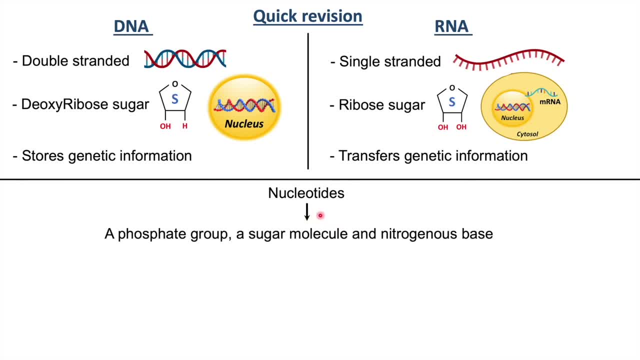 up of nucleotides, and these nucleotides, um, contains a phosphate group, a sugar molecule and a nitrogenous base and, furthermore, this nitrogenous base. there are two nucleotides, two forms of nitrogenous base. one is purine and pyrimidines. purines are double member. 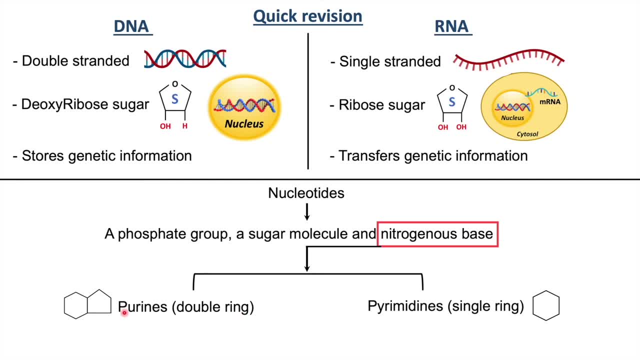 double ring and and like i like i said before, purines are shorter name and longer structure, pyrimidines longer name and shorter structure. that is six member ring and that means it's a single ring. purines contain adenine and guanine, whereas pyrimidines contain.